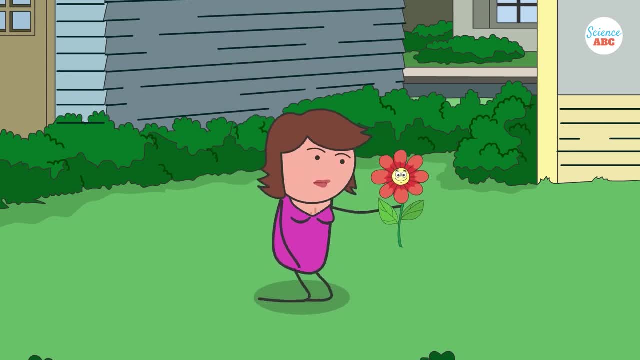 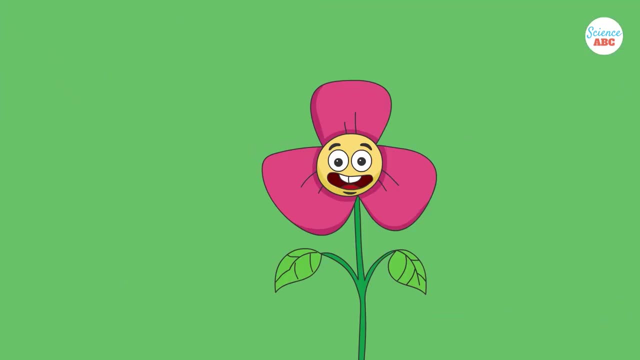 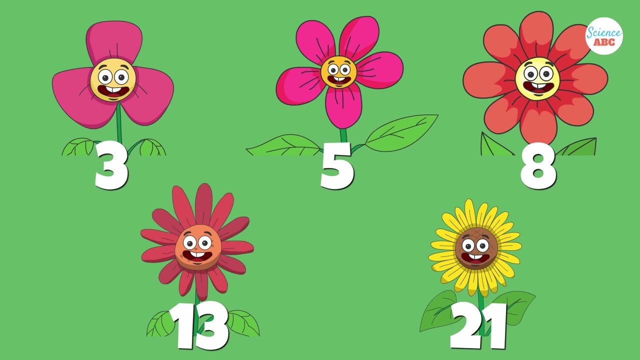 Have you ever counted the number of petals on a flower? If you counted them on a flower with petals all intact, you would likely discover that the number of petals is a Fibonacci number, that is, a number from the Fibonacci sequence. Many flowers have 3,, 5,, 8,, 13, or 21 petals. 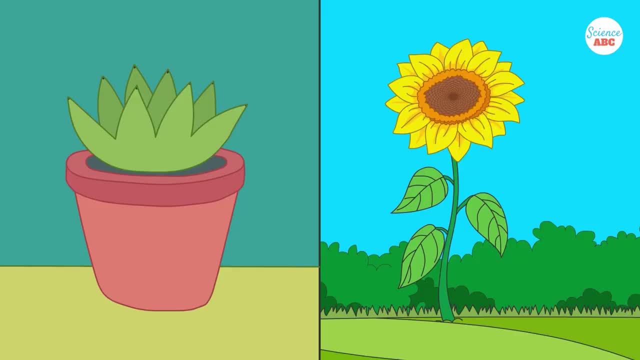 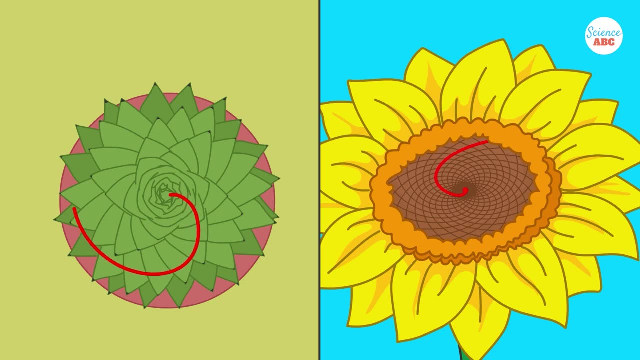 all of which are numbers in the sequence. The leaves of cacti and the seeds of sunflowers are arranged in both left and right-handed spirals. The numbers of seeds or leaves in these spirals are also generally in the Fibonacci sequence. We have two hands, both of which. 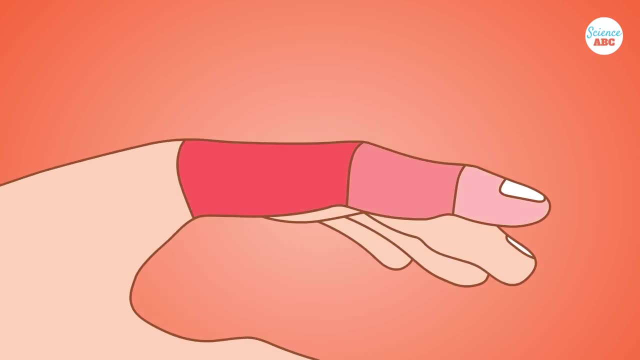 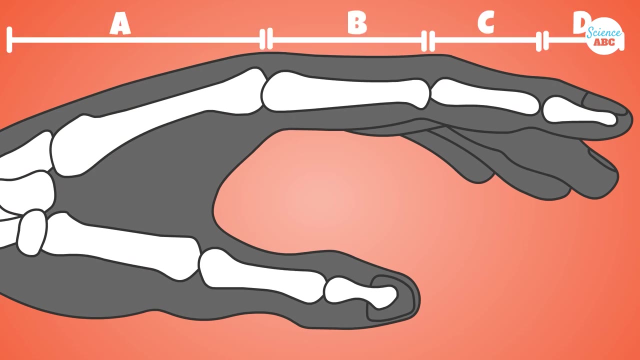 have five fingers, and each finger is divided into three parts. All of these numbers are also Fibonacci numbers. Moreover, the lengths of the bones in our hands also fit into Fibonacci ratios. So what's the Fibonacci sequence anyway, and why is it seemingly everywhere? The Fibonacci sequence is a series of numbers in which a given number is the result of adding the two numbers before it. So if you start with 0,, the next number will be 1, followed by 1, followed by 2, followed. 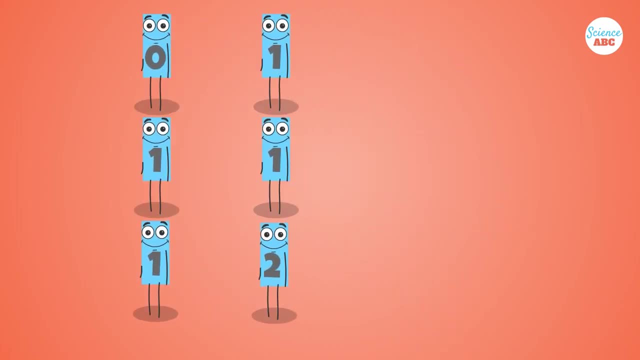 by 3, and so on. As you can see, every number in this series or sequence is obtained by adding the two preceding numbers. Individual numbers in this sequence are often referred to as Fibonacci numbers. Mathematically, the Fibonacci sequence is represented by this: 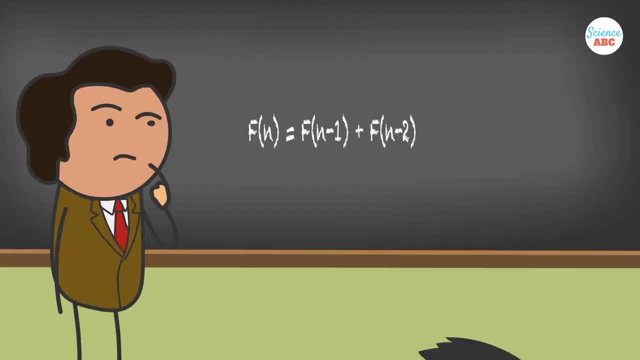 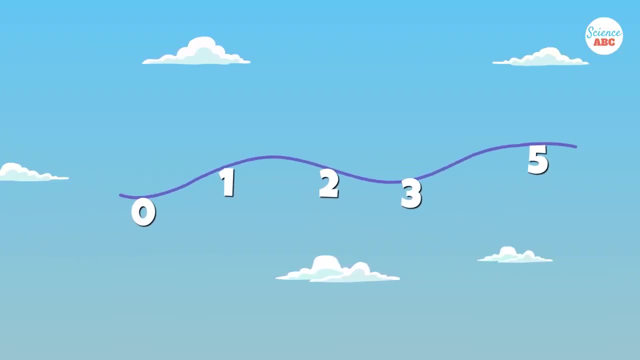 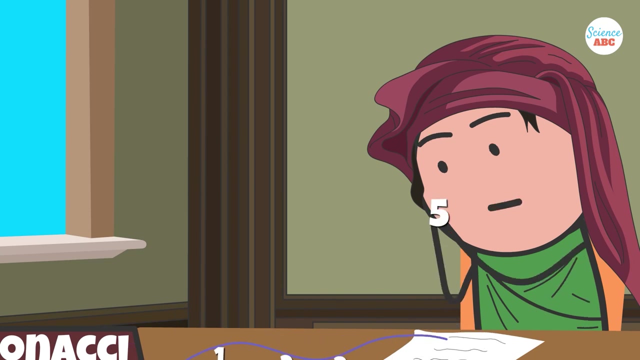 formula where n is greater than 1.. You can use this expression to find any nth digit in the sequence. This fascinating sequence is widely associated with the mathematician Leonardo Pisano, also known as Fibonacci. He hailed from the Republic of Pisa, which 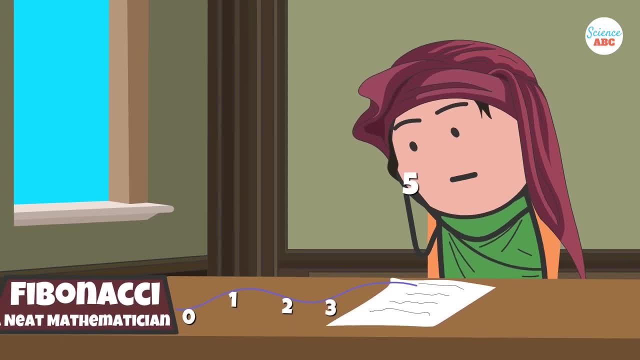 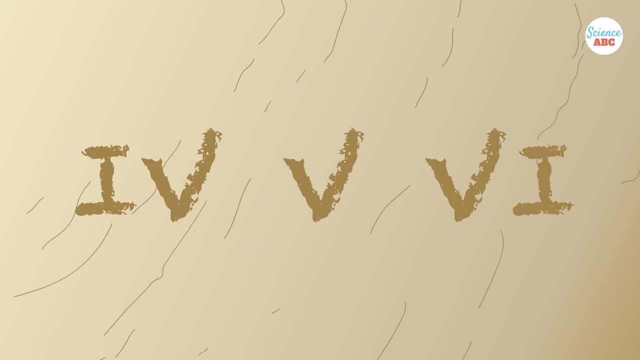 is why he is also known as Leonardo of Pisa and is considered to be one of the most talented mathematicians of the Middle Ages. At the time, Europeans were still using Roman numbers, while Hindu-Arabic mathematicians were using a different number system that was more robust. 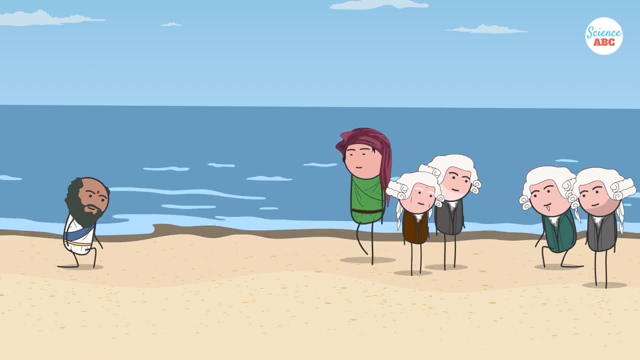 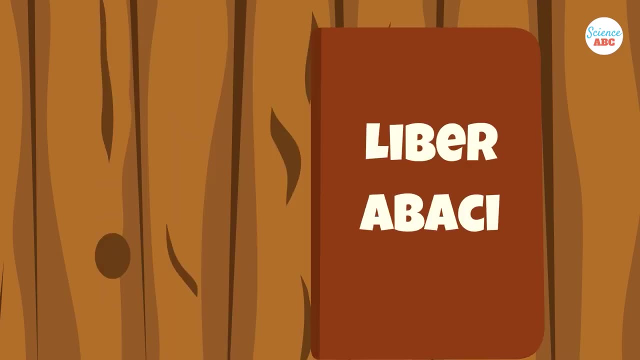 and efficient. Fascinated by the brilliance of the Hindu-Arabic number system, he decided to bring it to the Western world in 1202 through his now-famous book Liber Abhaki. In the book, he reviewed and compared the Hindu-Arabic numeral system with other systems, such as: 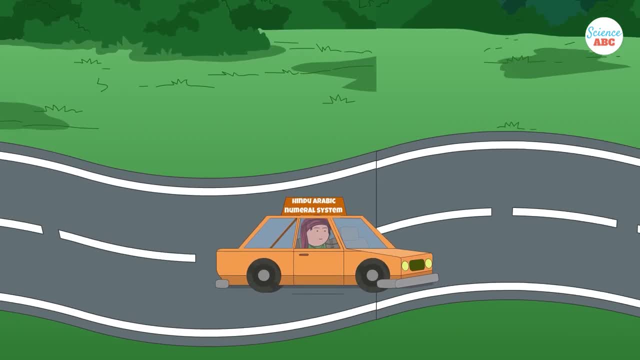 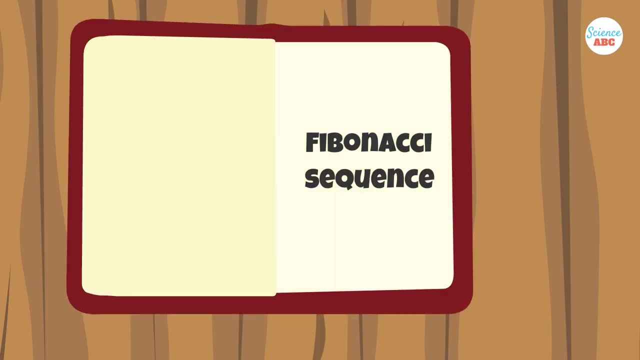 Roman numerals and described how using the Hindu-Arabic system made calculations faster and easier. Although his book contains the earliest known description of the Fibonacci sequence outside of India, it was described in ancient Indian texts by mathematicians as early as the 6th century. 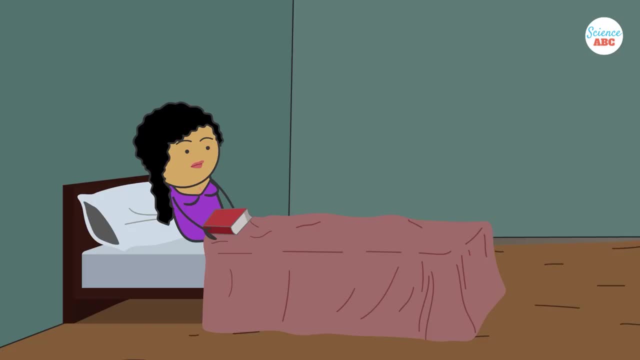 So what makes this Fibonacci sequence so special? To the uninitiated, this famous sequence may just seem like a series of numbers, but the Fibonacci sequence has been discovered and rediscovered in various forms, not only in mathematics but also all across the natural. 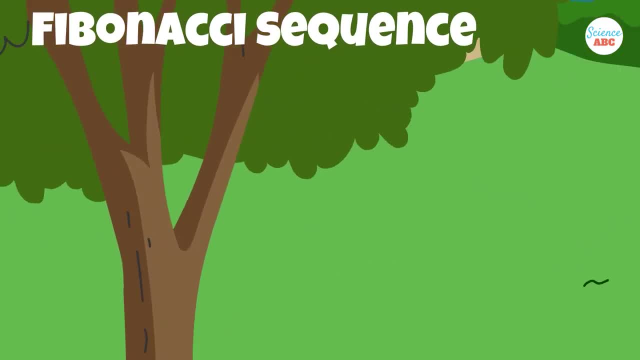 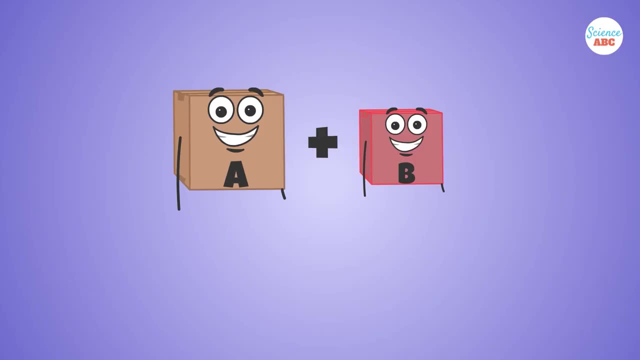 world and in our everyday lives. There's also another exciting offshoot of the Fibonacci sequence: the golden ratio. Suppose you have two quantities, A and B, wherein A is greater than B. Now add A and B and you get A and B. 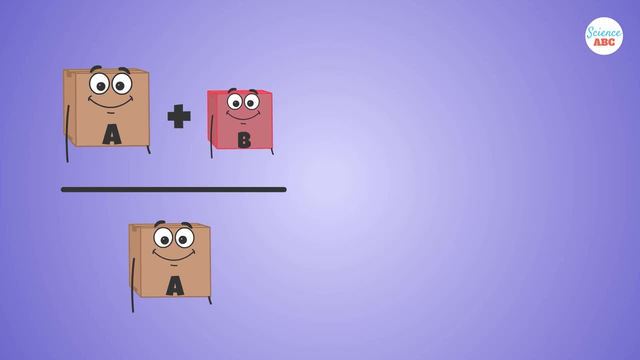 And divide that sum by A. If this ratio comes out to be equal to the ratio of A and B, then you can say that A and B have a golden ratio, which is represented by the Greek letter phi. Write down the Fibonacci sequence on a piece of paper and calculate the ratio using this. 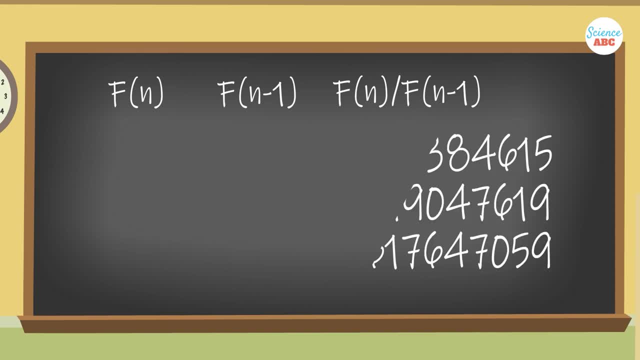 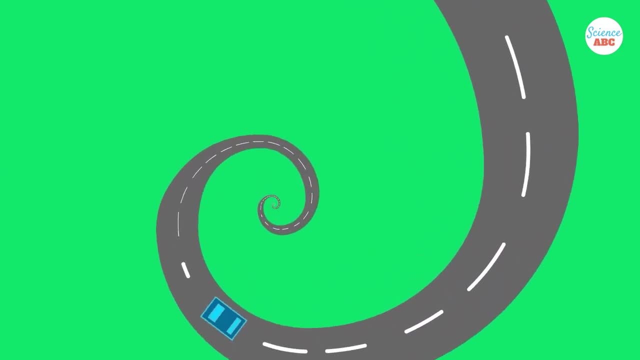 formula, You will notice that all Fibonacci numbers have the golden ratio, the value of which is close to 1.618033.. In geometry, when the golden ratio is applied as a growth factor, you get a special type of logarithmic spiral known as a golden spiral. Simply put, a golden 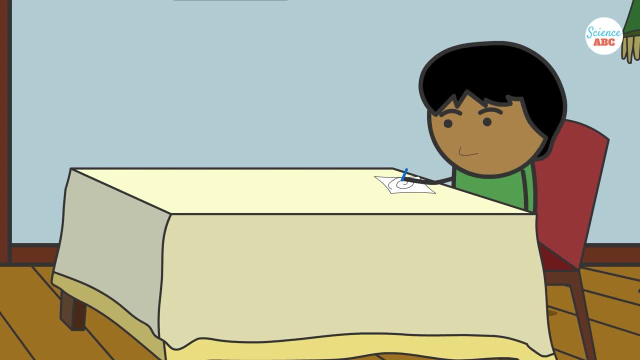 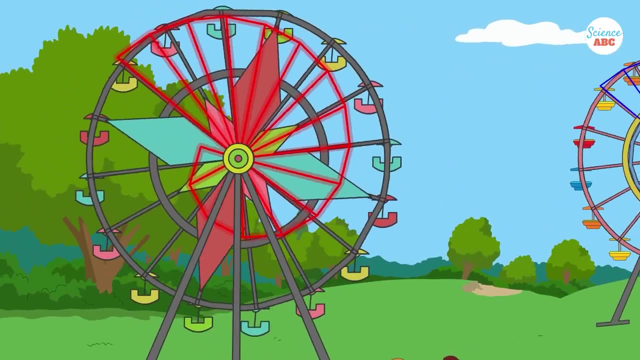 spiral gets wider by a factor of phi for every quarter turn it makes. You can find examples and manifestations of the golden ratio and golden spirals in countless places in your everyday life. Seashells are some of the most common examples of the golden spiral found. 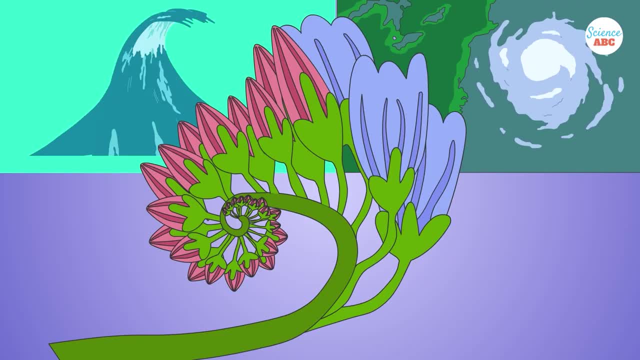 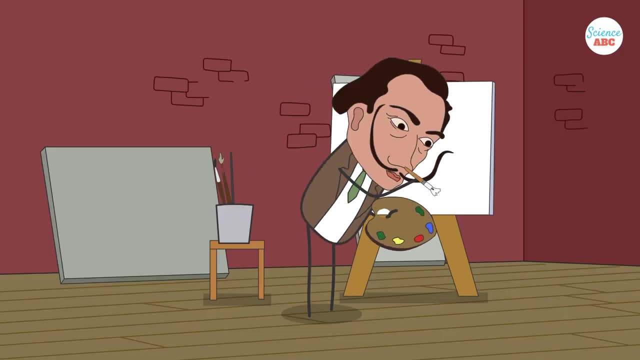 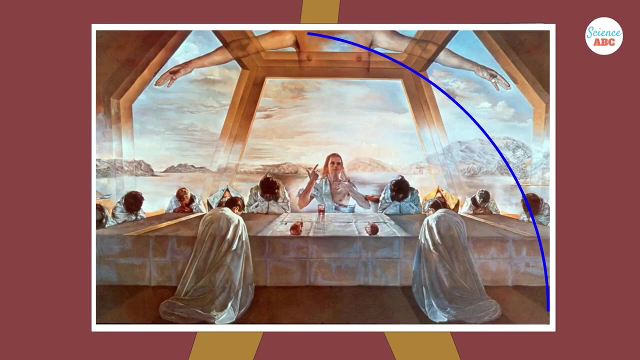 in nature, but ocean waves, hurricanes, flower buds, snail shells and spider webs are just a few of the other naturally occurring examples. Many artists use the golden ratio, or the golden spiral, in their creative works. Legendary painter Salvador Dalí explicitly used the ratio in his masterpiece, The Sacrament of. 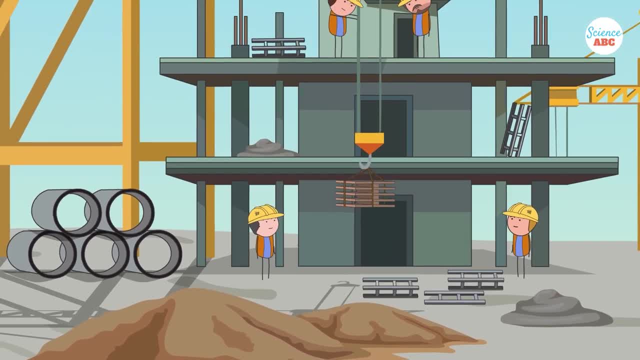 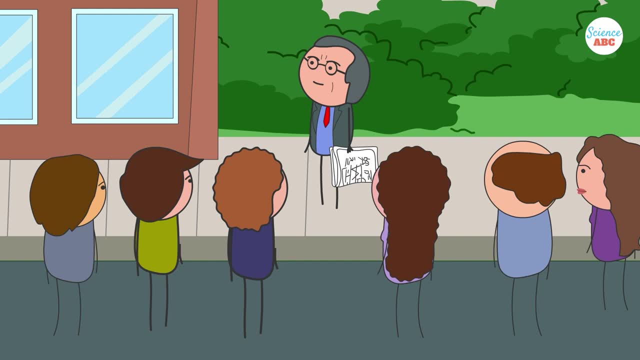 the Last Supper Architects also commonly use the golden ratio when designing buildings and other massive structures. Popular Swiss-French architect Le Corbusier, who is widely acclaimed as one of the pioneers of modern architecture, explicitly used the golden ratio in his modular